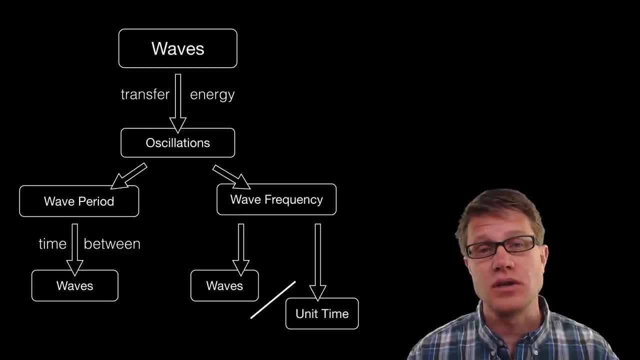 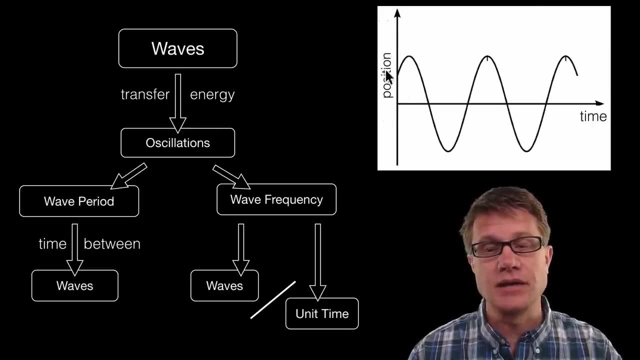 we are going to measure wave frequency in hertz, which is the number of waves per unit time. Now, if you are ever looking at a wave diagram like this, the first thing you want to do is figure out what are my axes labeled, And so the position is changing here. But 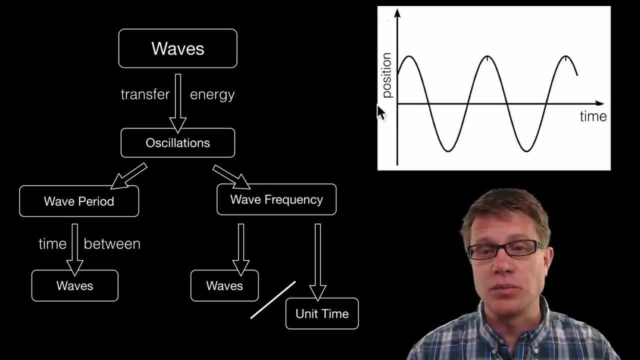 this is over time. Now you could also have wave diagrams where it is position here and position here. But since we have time on the x axis, if I want to figure out what the period is, I simply measure the distance between waves, And so I find one wavelength, So one. 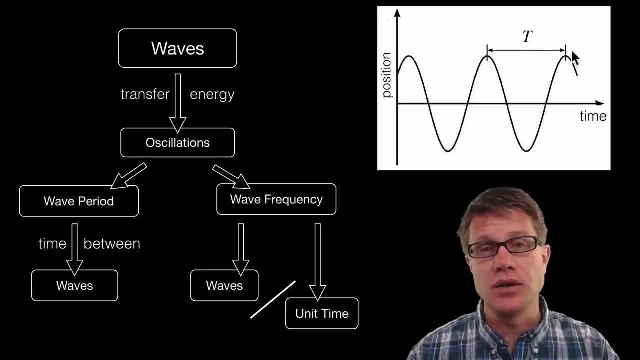 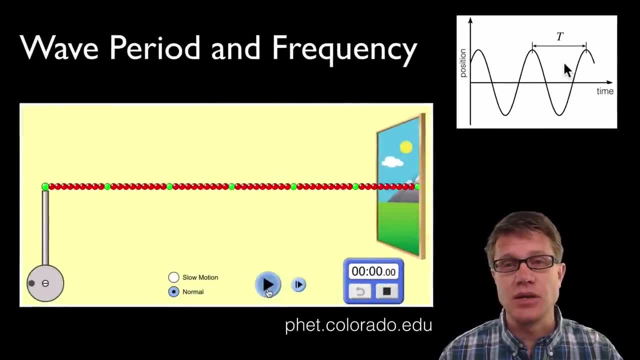 oscillation, And then the distance between the two is going to be the period, Or it is going to be the time. If I wanted to figure out the frequency, then it is simply the reciprocal of that. And so let's do a little simulation. This is a PHET simulation. What I am going to do. 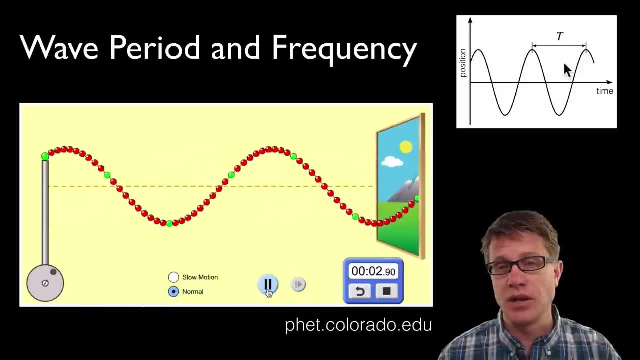 is generate some waves, And so those waves are moving from left to right, And so this is going to show us the position, But it is going to have a certain frequency And therefore a certain period. Now, a way to see that is to slow it down, Since we are looking at a 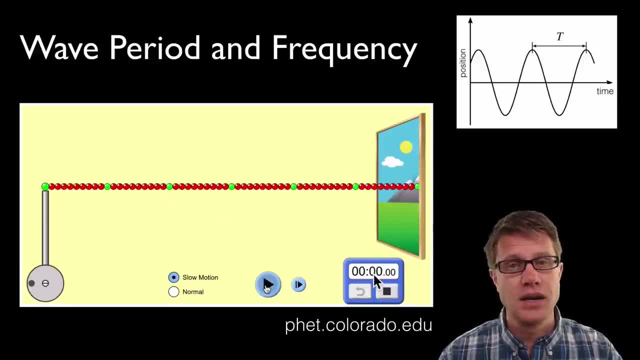 position of the wave over here. I have also added a clock, And so we can keep track of that time. And so we are going to create one wave, And so I am going to stop it after we go through one oscillation. And so what is going to be? 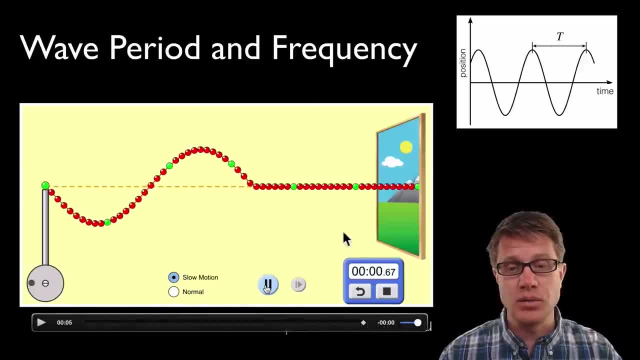 our period. Well, we have got the one wave here, But what is the period? It is the time. It is simply 0.67 seconds, And so that is the time distance between waves. We are just about to start another wave. Now, if I want to figure out frequency using this simulation, 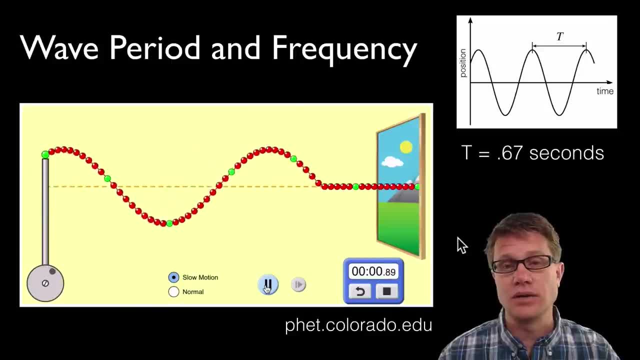 what I could do is just let that clock run until it gets to one second, So I am going to stop it here. So that is one second. And so how many waves do you see on the screen? Well, I see one and a half waves, And so our frequency is going to be 1.5 hertz. Now we 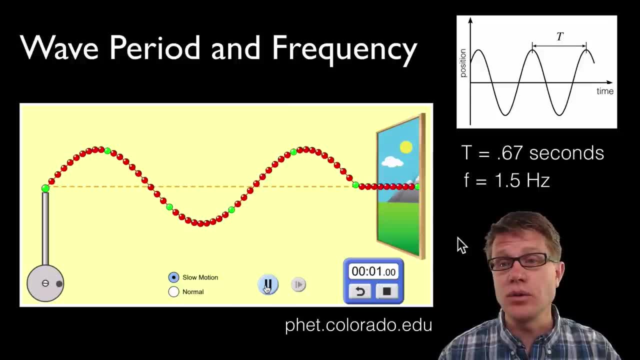 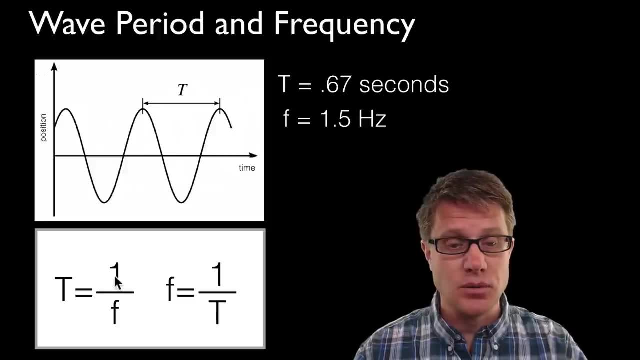 could have done it just by looking at the simulation, doing some experimentation, Or we could just do it mathematically. If we want to convert from 0.67 seconds into frequency, all you do is we would take that period that we calculated, 0.67 seconds. we take 1 divided.